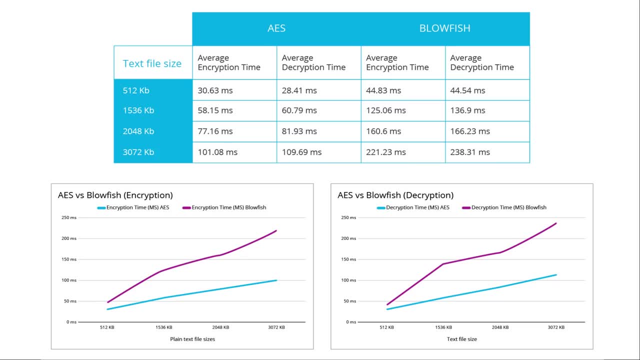 be accomplished by using ridiculously larger encryption keys that are more bits in length. Again, remember DES was only 56 bits in length. But the encryption and decryption times of this algorithm also had to be very fast and the algorithm had to be completely open source. 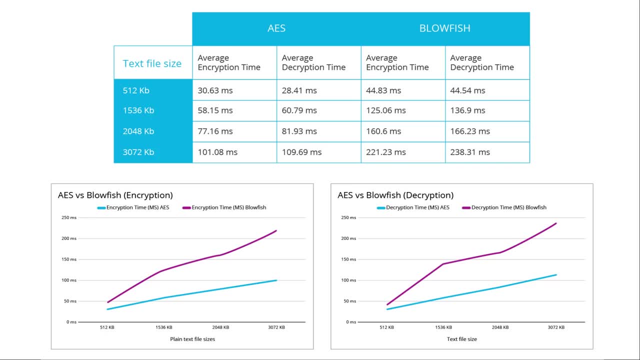 so that there's no reliance on security through obscurity. You don't ever want that to be one of the primary strengths of your encryption, to be the fact that just nobody knows it, because it's only a matter of time until some people find out. 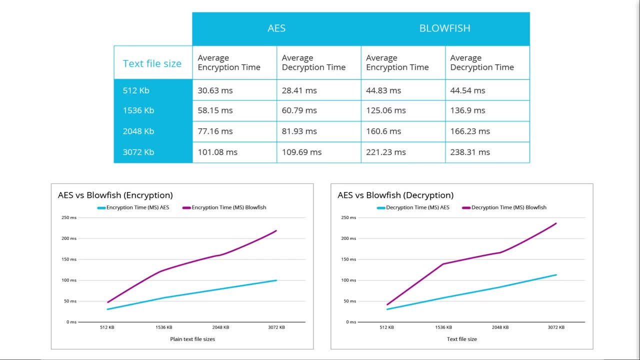 and then your encryption is going to be broken. And, more importantly, it has to be open source to make sure that there's no backdoor weaknesses that are built into the encryption to be maliciously taken advantage of later. So, out of the dozen or so submissions, 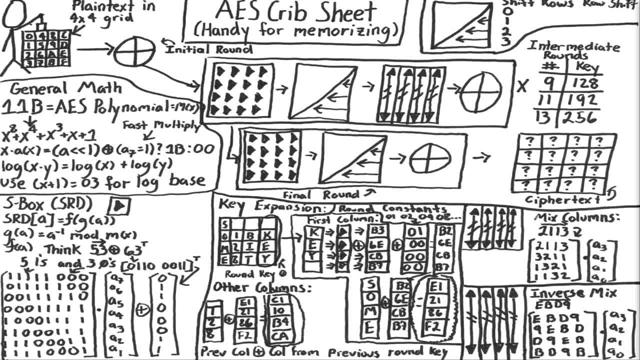 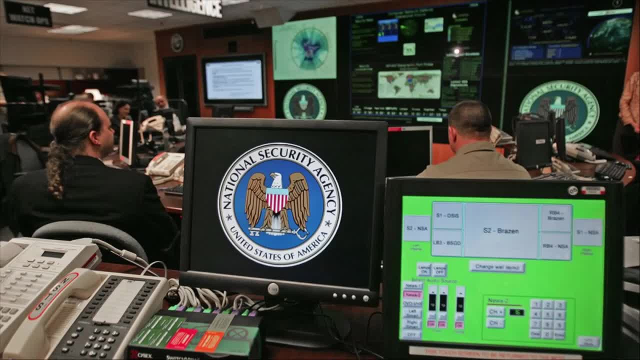 the Rheindahl cipher emerged victorious, which was the original name of AES. It took on that name in 2002, and then became really popular in 2003 after the NSA- one of the brightest, glowing government agencies- approved AES for encrypting top secret government information. So now AES. 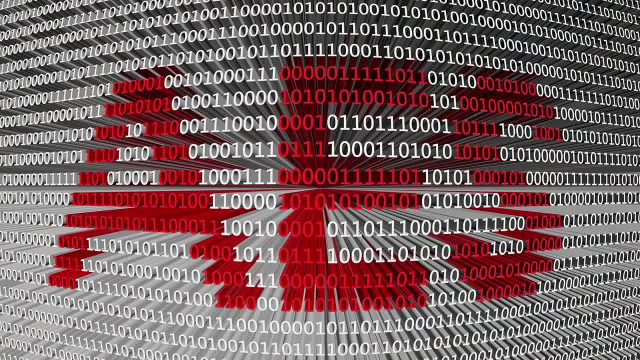 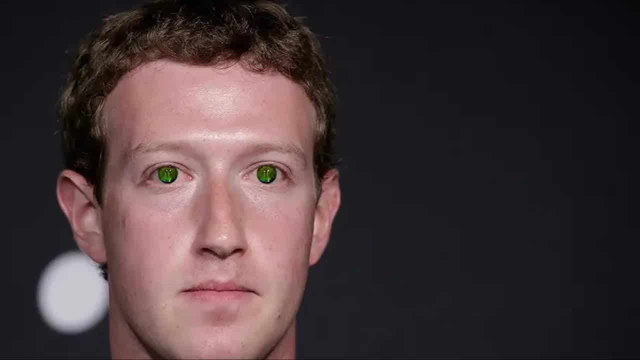 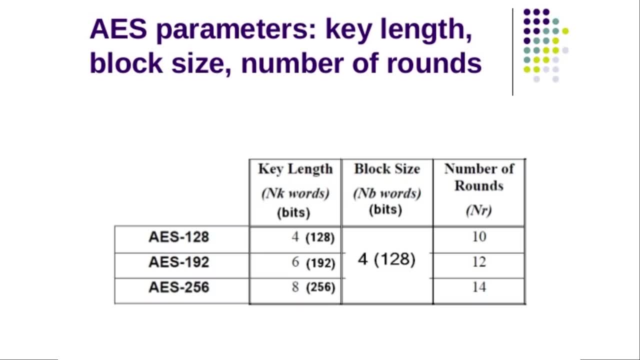 it has made it to the top. It has become the industry standard for encryption used by corporations, the government and you. I mean, if it's good enough to encrypt information about aliens and the misappropriation of tax money, it's good enough for encrypting your emails, right? So how does it actually work? 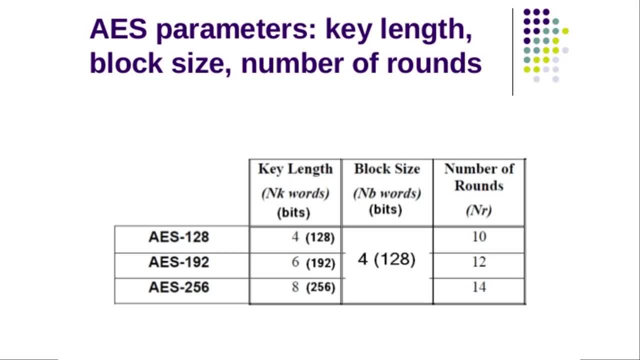 AES uses a 128-bit symmetric block cipher, So it takes 128 bits of a message or a file- you know whatever kind of data that you're encrypting- and it encrypts it into 128 bits of ciphertext, with a key that can be either 128,, 192, or 256 bits. 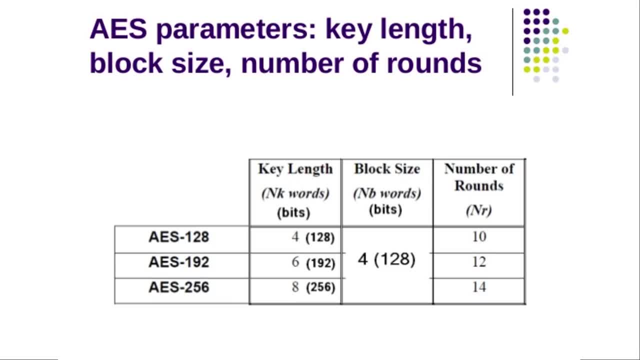 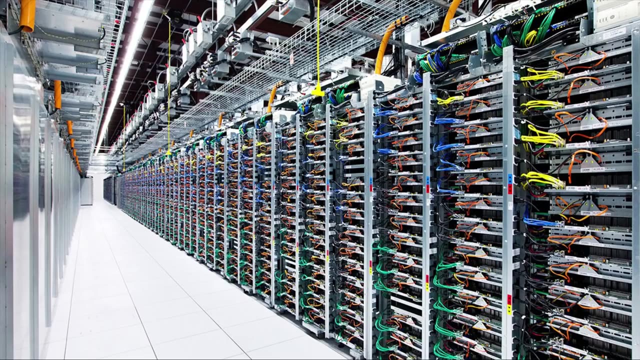 So the more bits that the key is, the more secure it is. Although don't feel bad if your browser or application that you're using has only implemented AES encryption with 128-bit key sizes, because that's still pretty hard to brute force. There's literally a one in two to the 128th power chance. 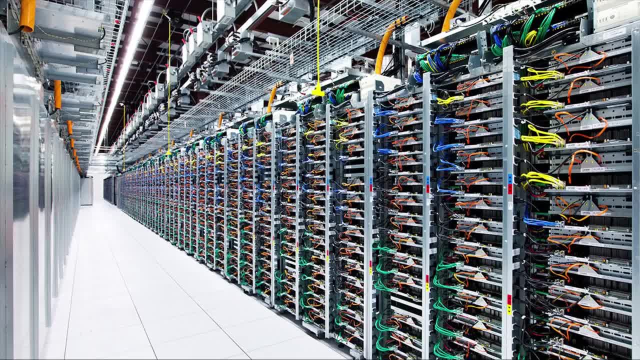 of guessing that correctly. And to put that in perspective, you could have 10 million computers that are all guessing 10 trillion times more than the average computer that you're using. There's a million different keys per second which, by the way, only supercomputers can really do. 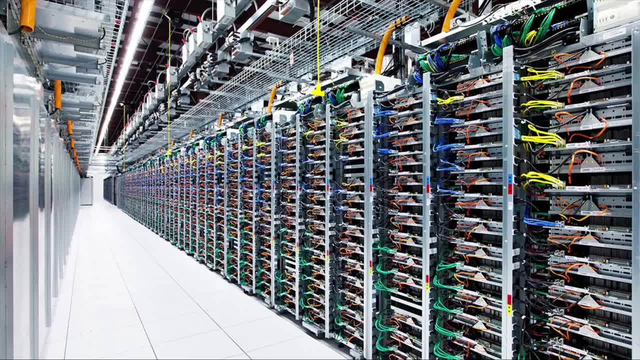 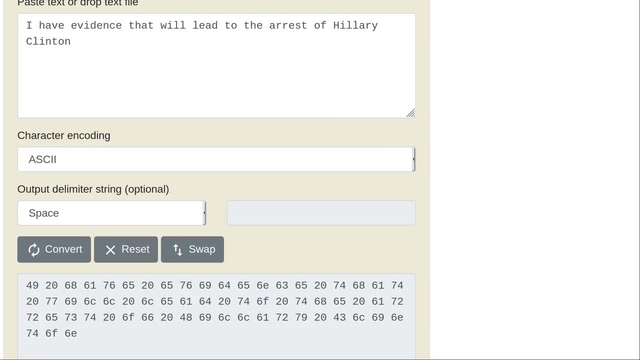 You need about 10 petaflops to get that many AES checks a second And it would still take them 107 billion years to guess every possible combination. So AES-128, still pretty secure. Now what AES does when it encrypts your message. 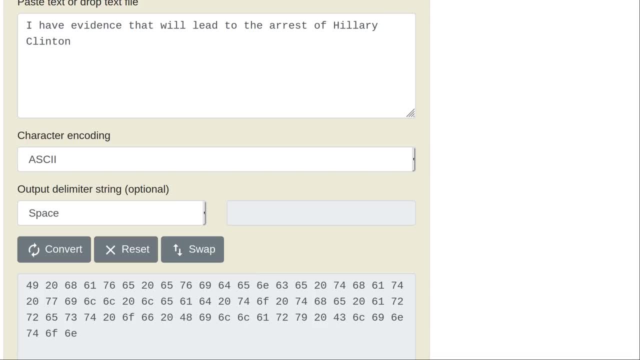 you, of course, start out with plain text data, which could be, like I said, text, video, audio, whatever, And then you convert it to hex, or you can convert it to binary, Either one, It's just. you know, it's fairly easy to divide them up into blocks. Hex is just easier to write. 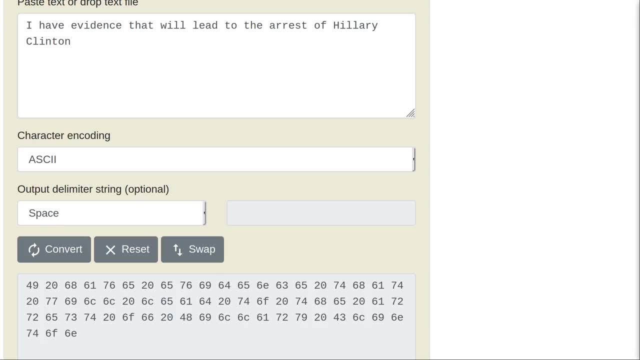 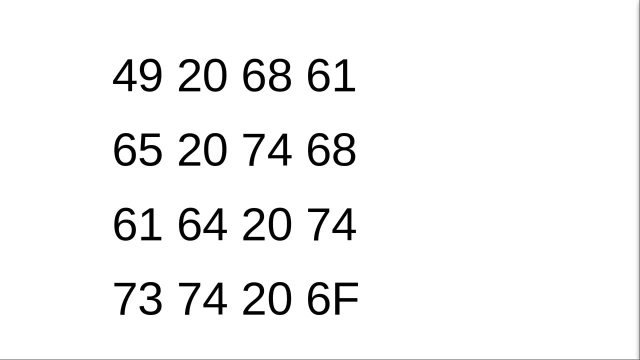 So our message is then split into 128-bit blocks that have four rows and four columns, And each entry is going to be two of those hex characters, which represents one byte, So it's going to be for 16 bytes, And then you're going to have to divide them up into blocks And then 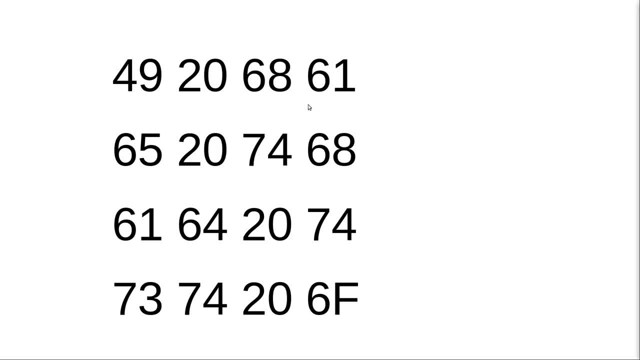 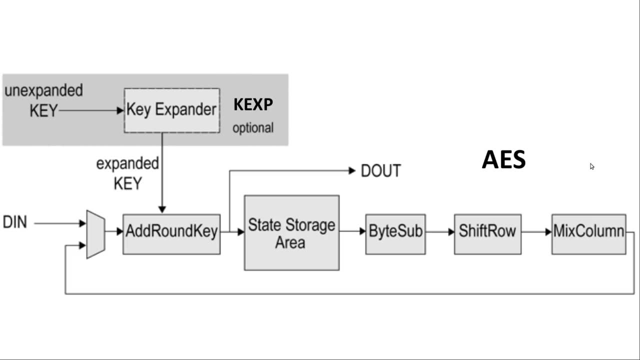 you're going to have to divide them up into 16 bytes in total or 128 bits. Now remember that this block size is always going to be the same. each chunk that it's taking out of your message, It's the key size. that can be different with AES. So next there's going to be a certain number of 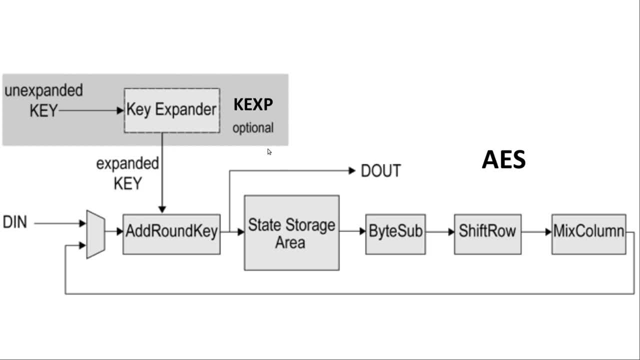 round keys that are created from the cipher key that you created when using the AES key schedule. So we'll go over what the round keys are in a moment, But you can think of them like a bunch of mini keys that are just derived from the original one. 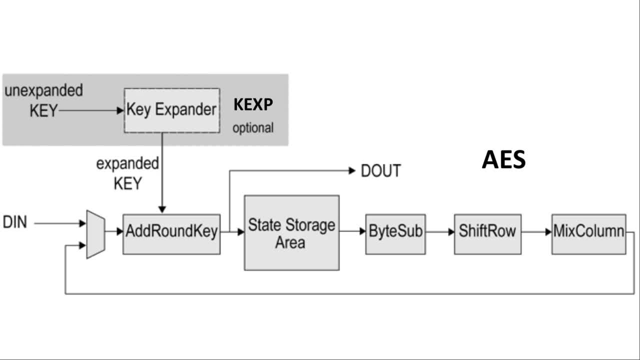 except each of these keys are not that small. They are each 128 bits And we're basically going to do a for loop over each of those different blocks that were broken out from your original data. So for each block of 16 bytes of data, combine it with one of the round keys by doing a bitwise. 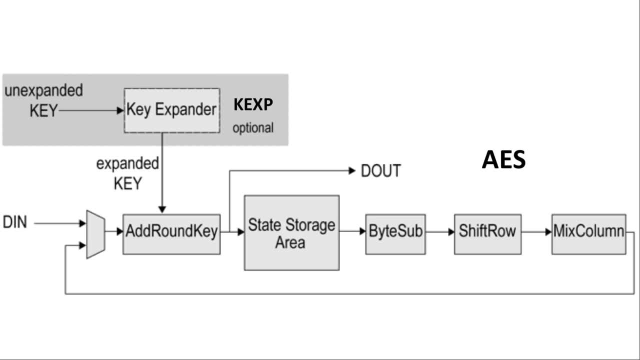 XOR between the bytes of the block and the bytes of the key, Then we're going to do some math on that block input combined with the key to further obscure it. Because if this was just raw hex combined with an encryption key, it would probably be pretty easy to sort the message out. 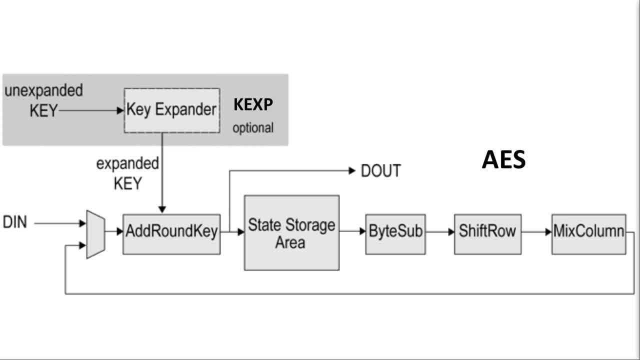 So the math that we're going to end up doing is a byte substitution And then we're going to mix up all of the rows and columns. So first we're going to shift the rows and then mix the columns- The byte substitution that's going to convert every byte into a different value. So AES is 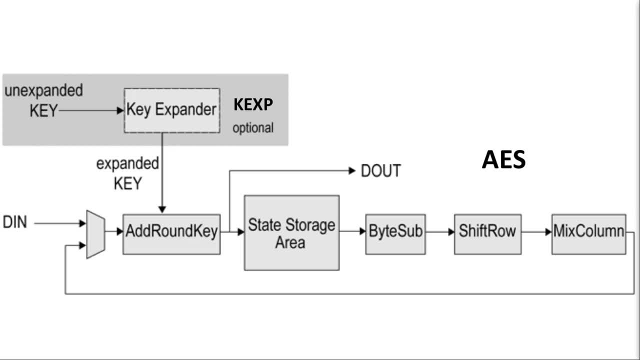 going to define a table of 256 different values, which is the amount of possible values that a byte can store. So, essentially, each value of the block is going to be changed to another one, And the function ensures that no byte is going to be replaced with itself with the same value. 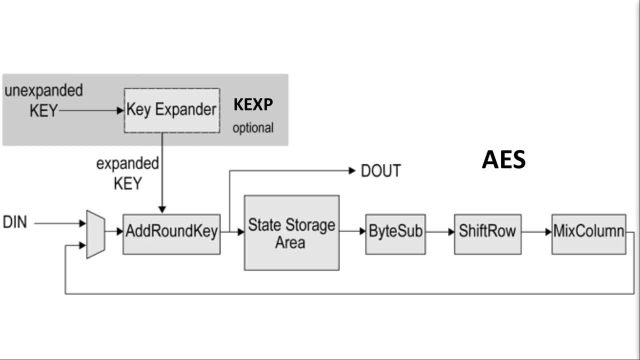 And this function is basically just a lookup table, So the implementation is actually very fast again as far as encryption and decryption times go. So then each row, So then each row, to be rotated to the left by an incrementing number of bytes. So zero for the first row. 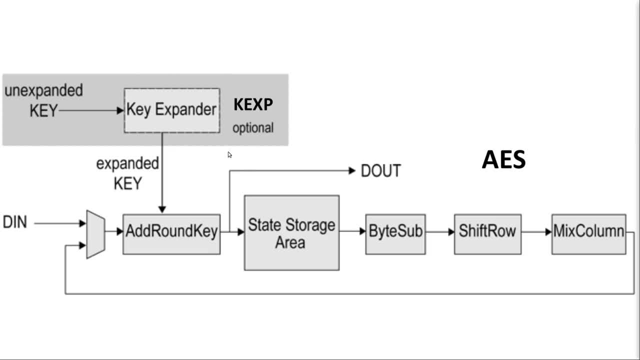 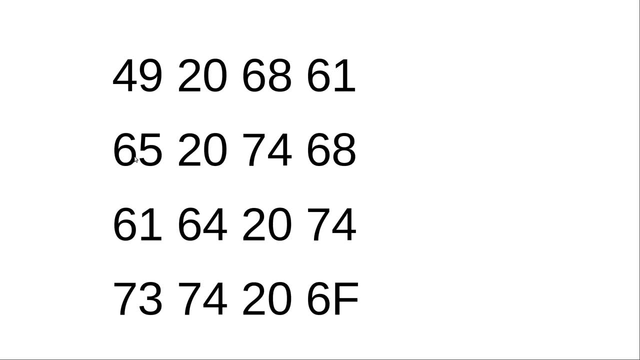 one for the second, two for the third, and so on. These bytes will also wrap around. So, for example, the 40, or the 65, rather, is going to be put into the position of the 68. And these are going to move over to. so, basically, the 61 is going to be in the place of the 20. And the 64. 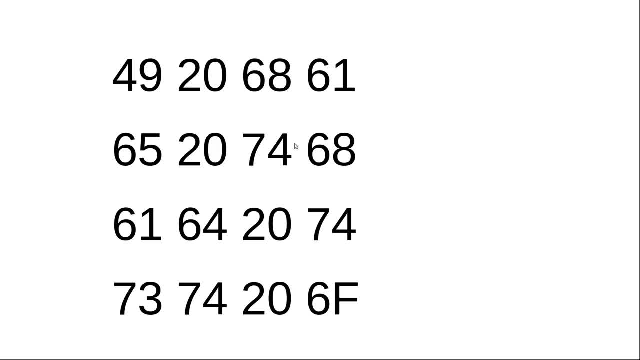 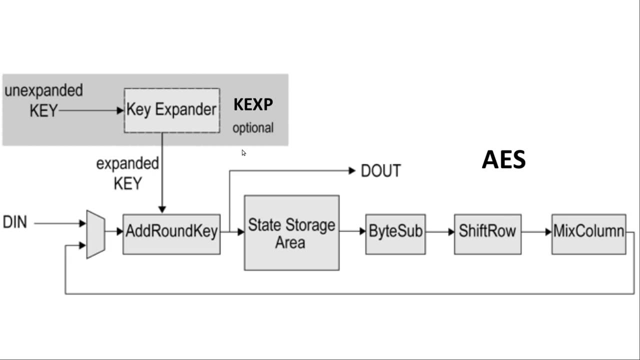 would be in the place of the 74. And then, finally, the mixed columns, which is the most complicated step, but it involves taking each column of the state array and then replacing it with a new column that is computed by a matrix multiplication. So it's basically just a lot of manipulation. 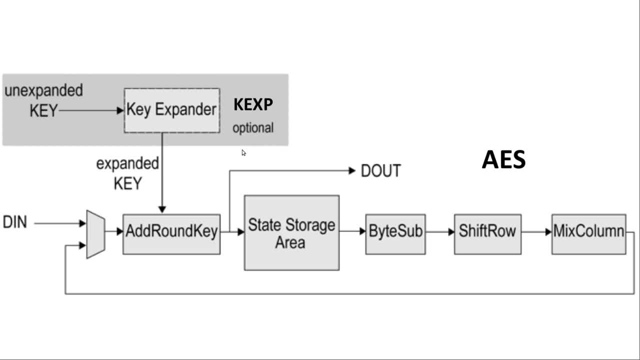 which essentially changes all of the values of the bytes and then changes all of their positions around to really jumble up all the data. And it would already be really hard to undo this, especially since the keys that you create at the beginning are kept a secret. 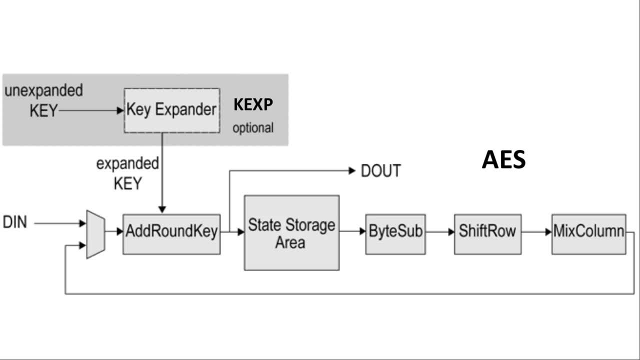 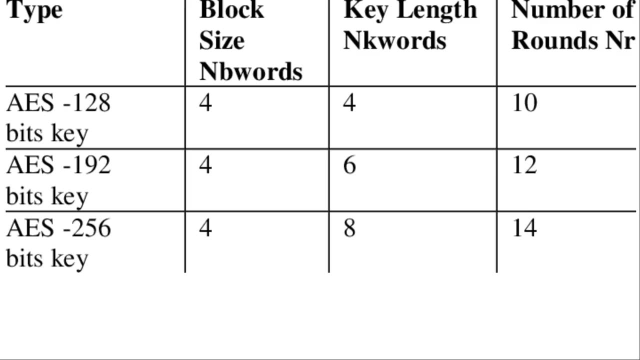 and those are essential to properly doing the algorithm. But these mixing up steps, these are going to be repeated a number of times and that's going to be determined by the key size that you choose to use. So 128-bit keys are going to repeat the process for 10 iterations by default. 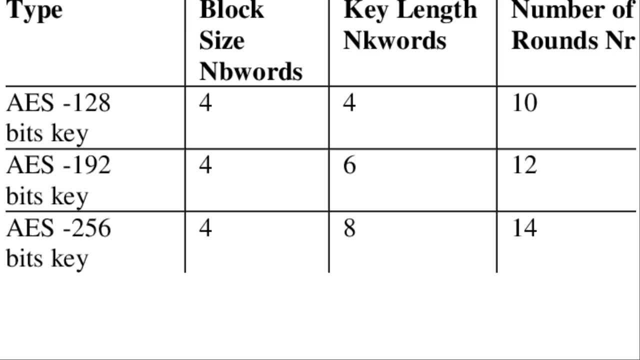 192-bit keys are going to repeat it for 12, and 256-bit keys are going to repeat it for 14 rounds, And during each round, a different round key is then going to be plugged into you. So the process repeats, starting off with XORing and the result from the last iteration. 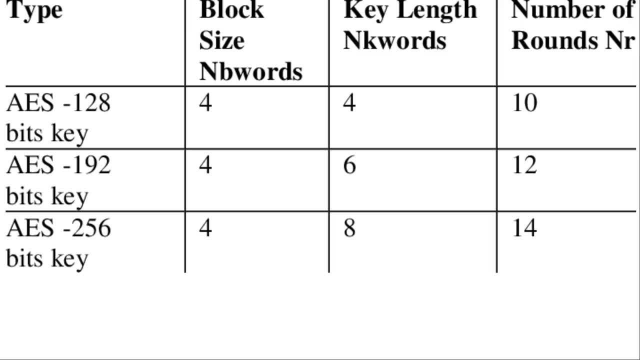 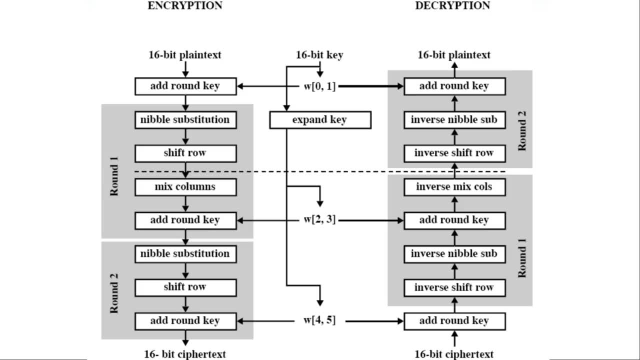 with the round key And then, on the final round, the process is repeated, except for the mixed column step, And when the data needs to be decrypted, we just do the inverse of the math and the movements that we did during the encryption for the same number of rounds. 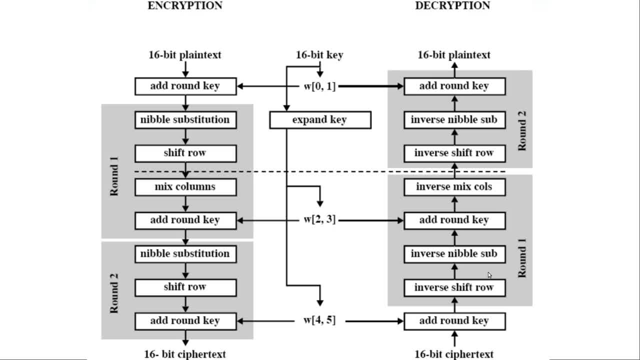 And, of course, nobody knows your encryption keys, so they can't access the data that is protected by it, at least not through cryptanalysis, which is very important to remember. It doesn't matter if you're using AES with 128-bit or 256-bit keys, because a hacker isn't going to attack the 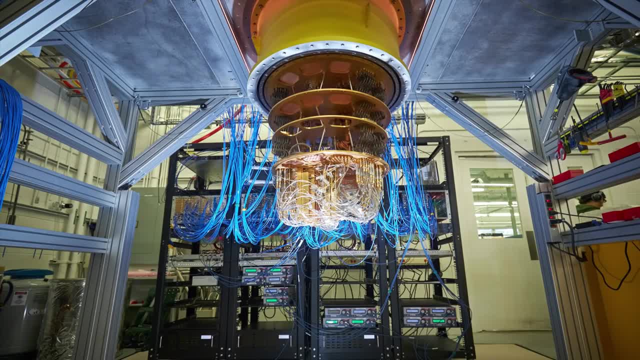 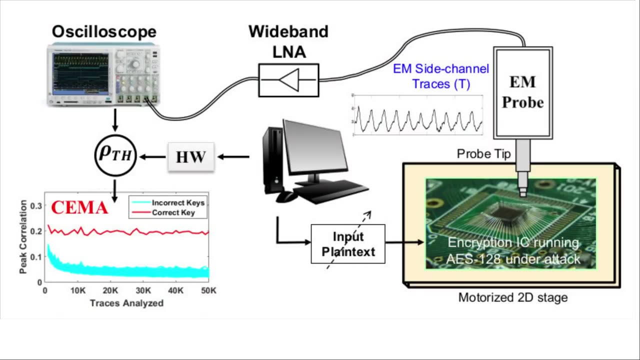 structure of AES itself. It's impossible to break that, at least until general-purpose quantum computers become a thing. So what a hacker is going to do is they're going to attack the weakest link in your security, which is either going to be an attack on the implementation of AES, if it's being implemented. 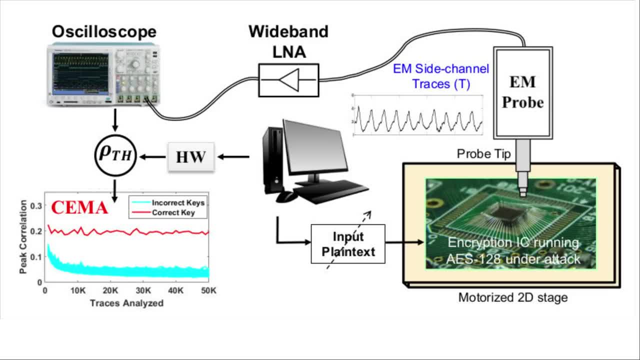 in software improperly and whatever application you're using or through a side-channel attack. if the hacker has hardware-level access to your system, they might be able to figure out what the encryption keys are from the cache. But what a hacker is realistically? 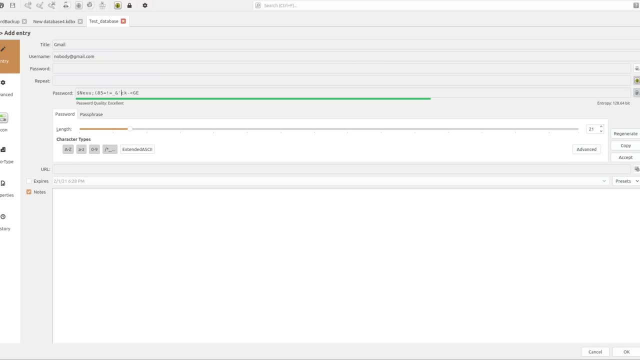 most likely to target is the password, So it doesn't matter if you're using 128-bit or 256-bit key sizes. if your password doesn't have a significant amount of bits of entropy, then guessing it is going to be easier, And if you're not using a password manager, I 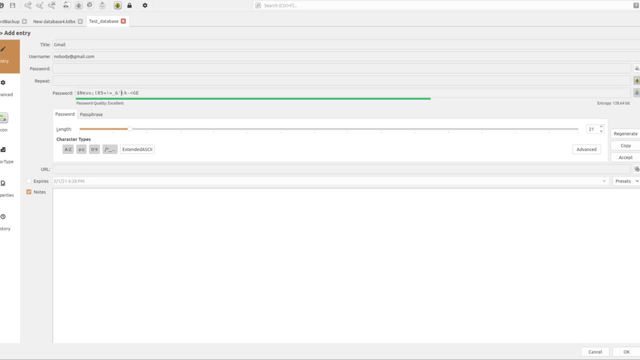 can pretty much guarantee that your password doesn't have very much entropy, because here is an example of one that just has 128 bits of entropy. So this is, you know, roughly the same as the smallest key size that you can use in AES, and it's still 21 characters.